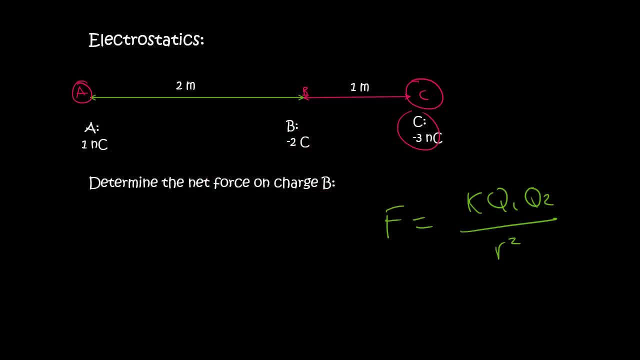 the same approach in this question. So let's have a look at the effect of A on B. So I'm going to say FAB equals to K, which is 9 times 10 to the 9, times by its charge. Now its charge is 1 for A and remember, when there's a N, then you have to use 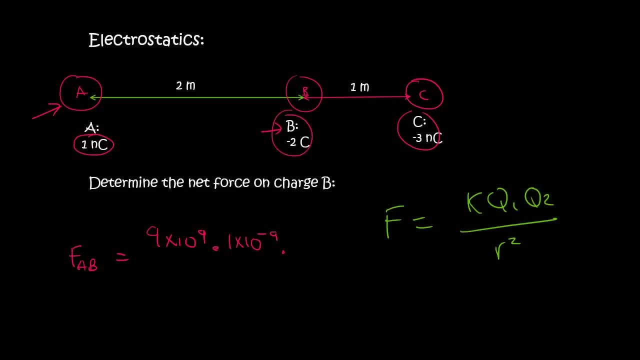 10 to the minus 9.. Then if I look at B, its charge is minus 2, but I don't put the minus in the calculation. The distance between A and B is 2, and then always remember the square, And so the 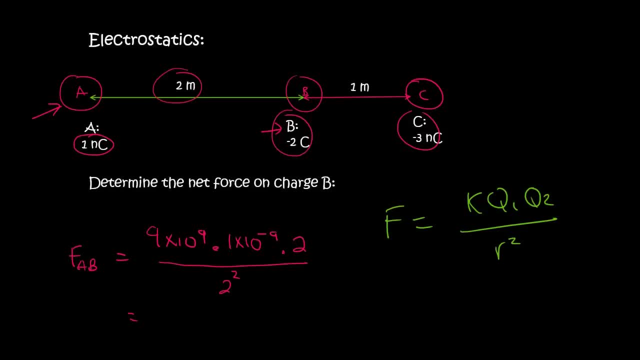 force of A on B is the following: We get 4.5 newtons. Now we are looking at B. We want to know what's happening to B. So A has a charge that is positive, B has a charge that is negative. So they'll definitely attract. 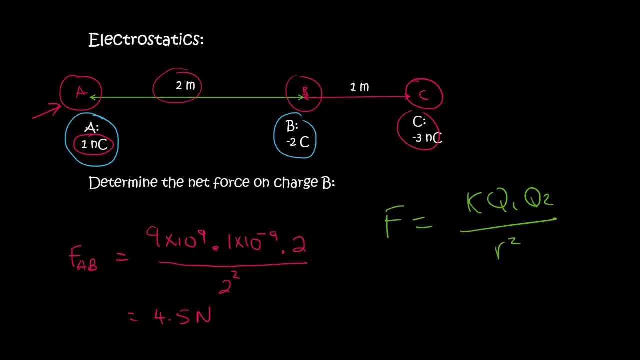 each other. So what does that mean for B? Is B going to move left or right? Well, well done if you realize that B will move left. But Kevin, what about A? A will move to the right, That's correct. 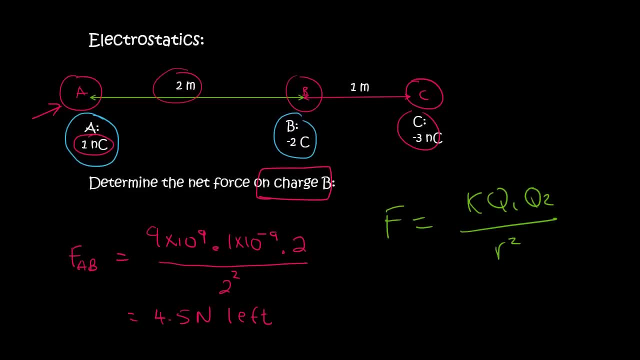 but remember, this whole question is about charge B. Okay, so we've done FAB, Now we need to look at the effect. So I'll say FAB, and that's going to equal to 9 times 10, to the 9, multiplied by B's charge. 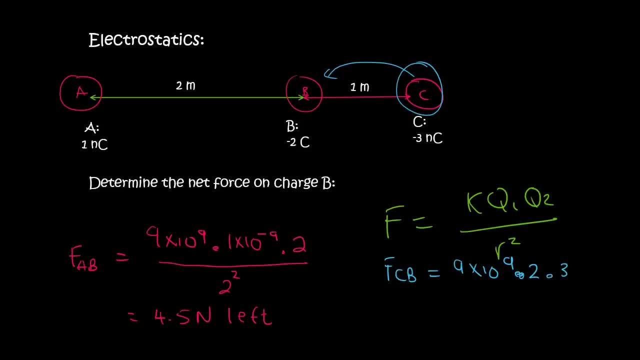 which is 2, multiplied by C's charge, which is 3, but it's got an N over there, so it'll be 3 times 10 to the minus 9.. The distance between them is 1 meter, and then square, And so if you do that, 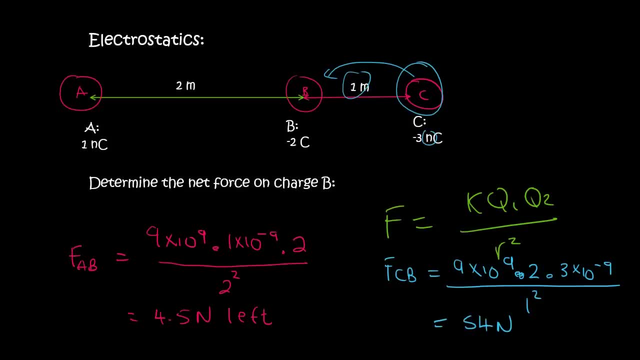 you would end up with 54. And what will C do to B? Well, B is negative and B is negative, so they're actually going to push each other away. So that's going to push B to the left and B will push C to the right. But we don't care about C because this: 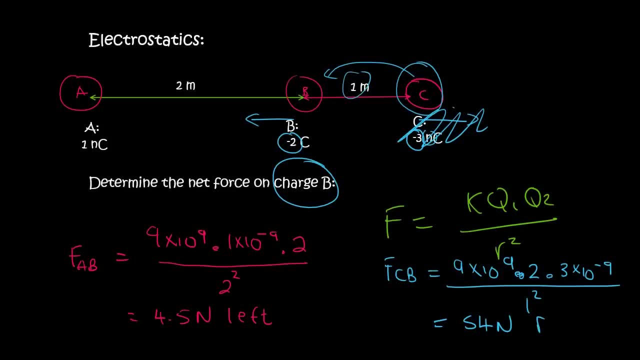 whole question is on B, So that's going to cause B to move to the left, And so both A and C are going to cause B to move left, And so to find the net force, we can just add those two together. If they were in opposite directions, well then we would have to do the same thing, So we're going to 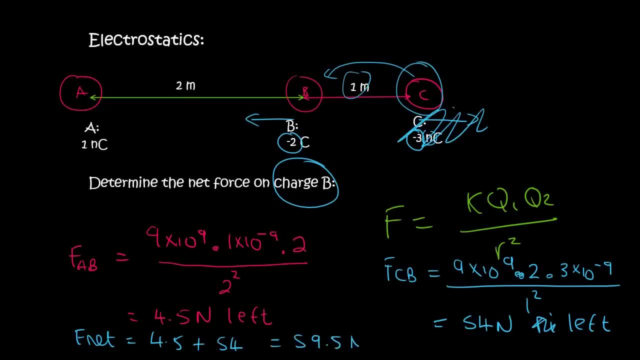 have to do something different, And so that's going to give us 59.5 newtons- 58, Kevin, 58.5 newtons to the left And Kevin, what about the force of A on C? Guys, we're not interested in. 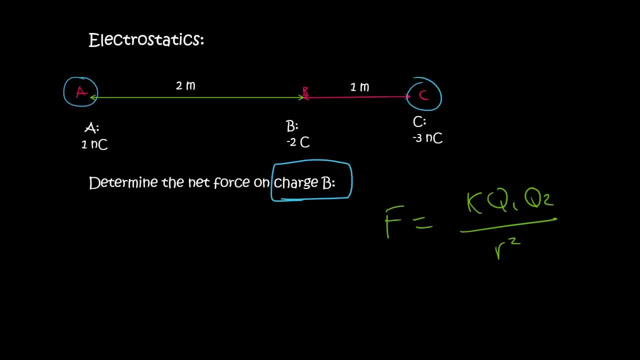 that because this whole question is about charge B. So here's another question. I've changed the order and I've changed the numbers and now I want us to work out the final charge on A. So now it's on this one. 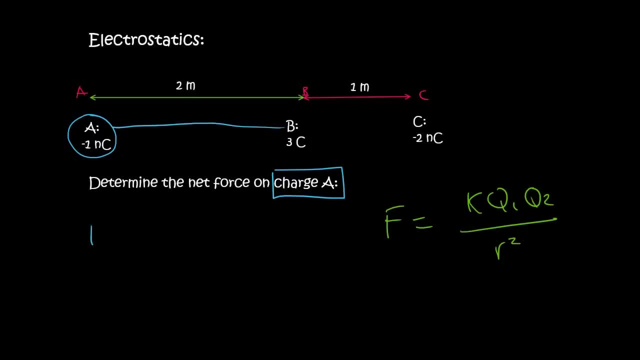 So what we need to work out is: how does B affect A? So let's do that first, So we can say: FAB equals to K, which is 9 times 10, to the 9, multiplied by A's charge, which is 1 times 10. 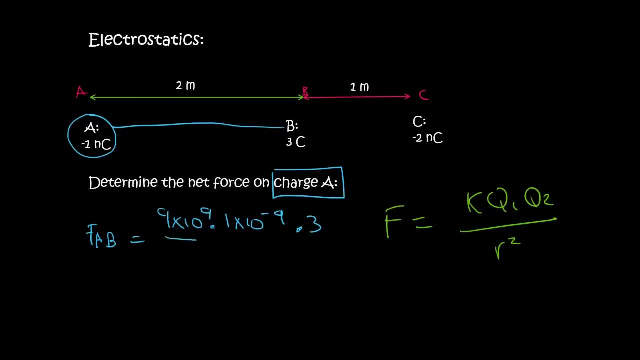 to the minus 9, multiplied by B's charge, which is 3.. And the distance between them is 2 meters, That'll be 2 squared, And so we can work that out, And that gives us 6.75 newtons. 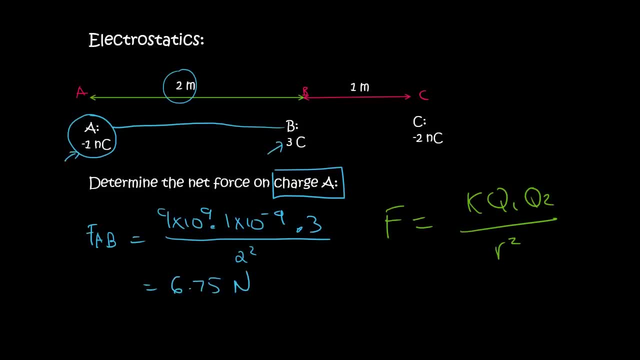 Now, A is negative and B is positive, So opposites attract. So what will A do? Well, obviously A is going to move towards B, B is going to move towards A, But we're not worried about B because this question is all about A. So it means A will. 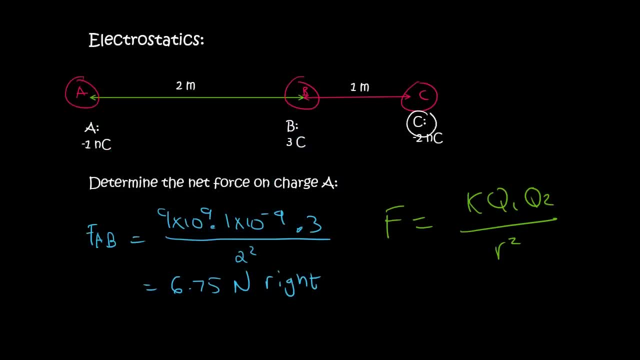 move. right Now we need to see how does C affect A? So we're going to go FB, no FAC, And so that's going to be K, which is 9 times 10, to the 9, multiplied by A's charge, which is 1. 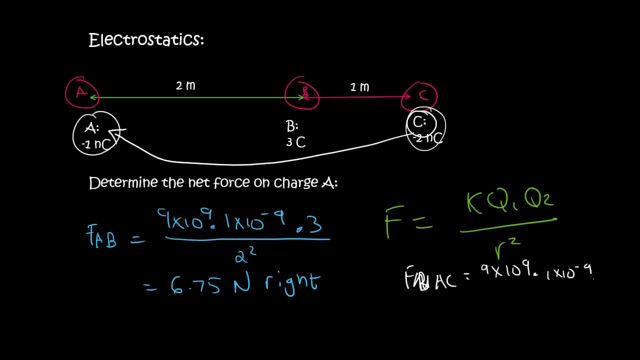 times 10 to the minus 9, multiplied by A's charge, which is 1 times 10 to the minus 9, multiplied by C's charge, which is 2 times 10 to the minus 9.. And the distance between them is 1. 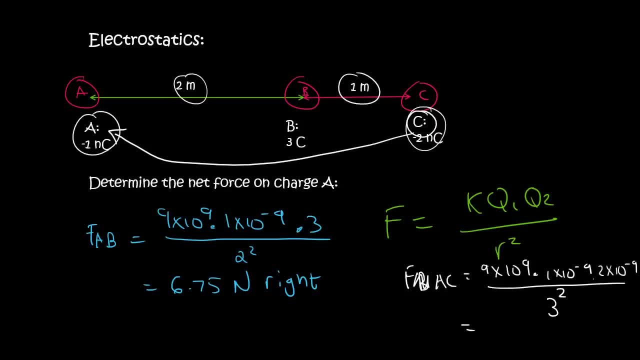 plus 2, which is 3 squared, And that gives us a very small value, 2 times 10 to the minus 9 newtons. Now, what would C do to A? Well, they're both negative, And so if they have the same charge, 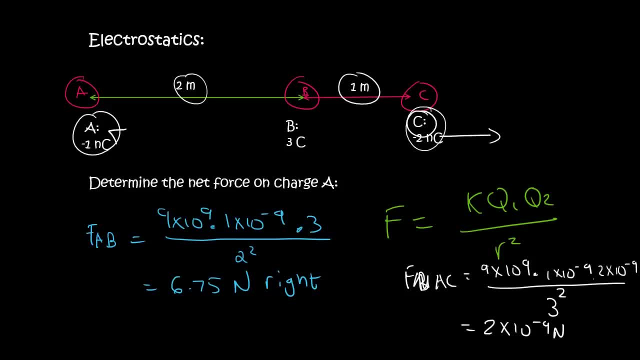 they will repel, So they'll push away from each other. So C would move to the right and then A would move to the left. So this is going to be left. Ah, so now we have B pushing A to the right and C pushing A to the left. So what's the overall effect? Well,